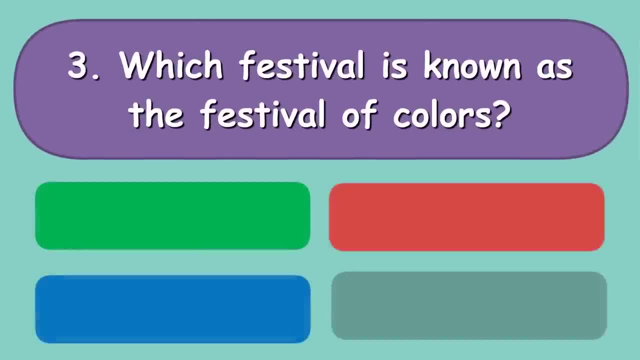 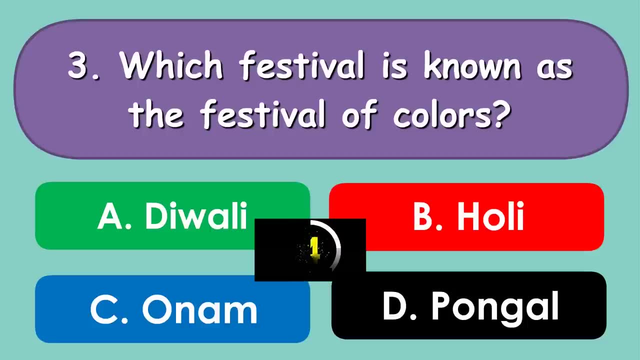 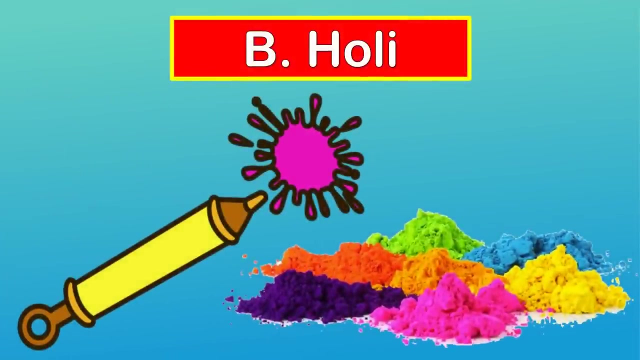 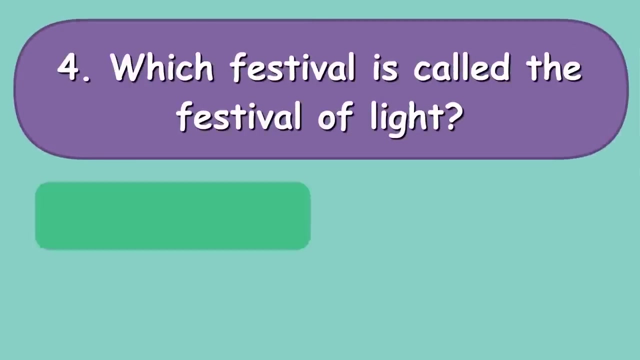 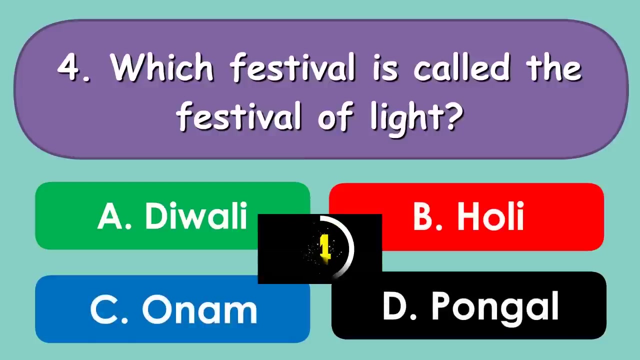 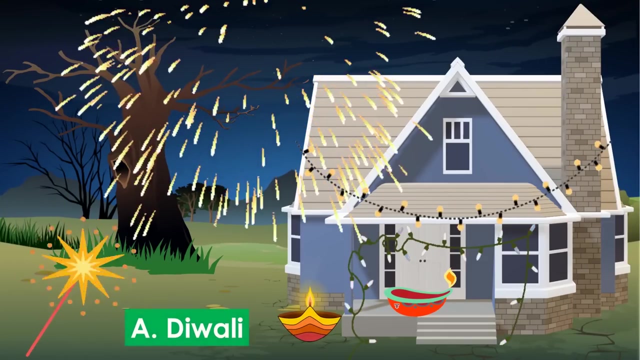 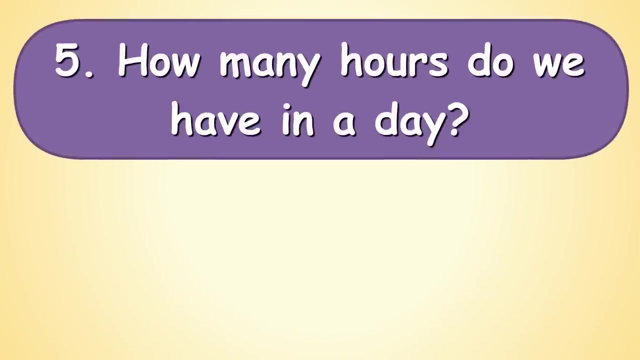 Which festival is known as the festival of colors? Holy is the festival of colors. Holy is the festival of color. Which festival is called the festival of light? Diwali, Diwali is called the festival of light. How many hours do we have in a day? 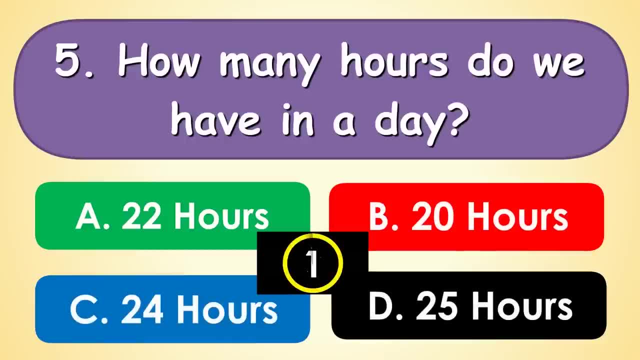 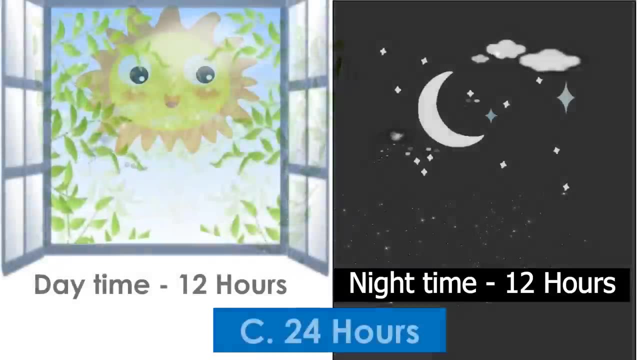 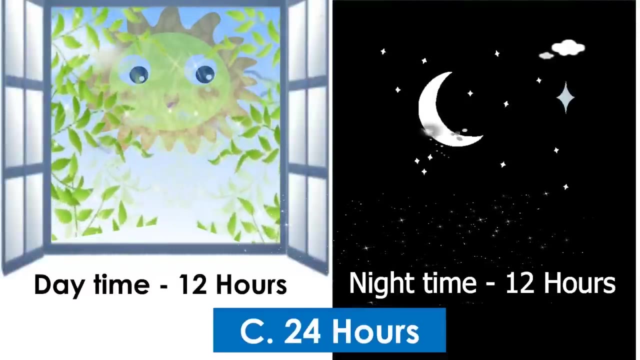 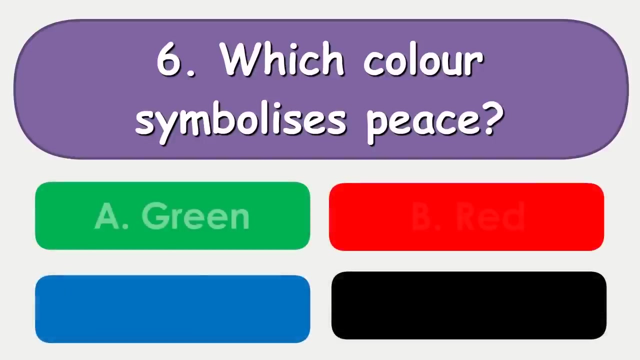 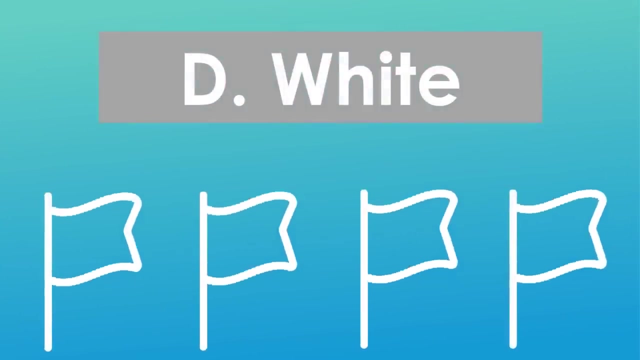 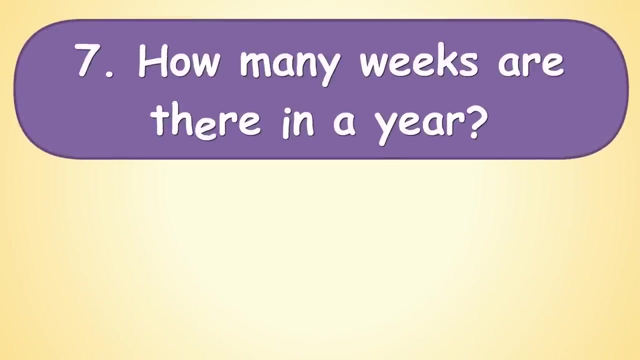 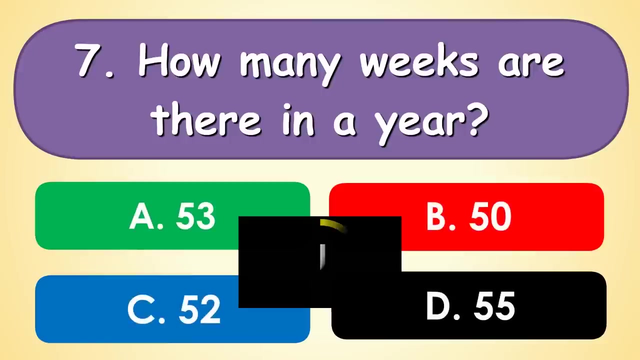 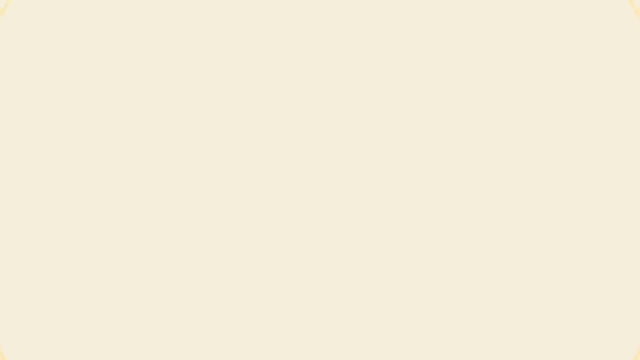 How many hours, How many hours? 24 hours, Daytime, 12 hours, Nighttime, 12 hours. Which colors in life? Peace? White color symbolizes peace. How many weeks are there in a year? 52 weeks. 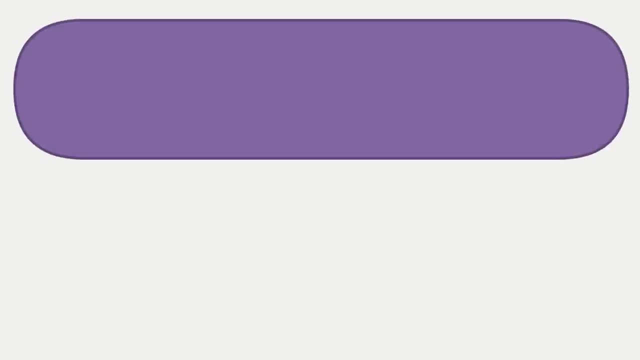 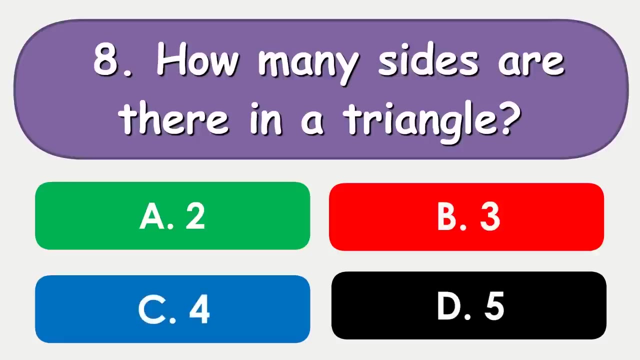 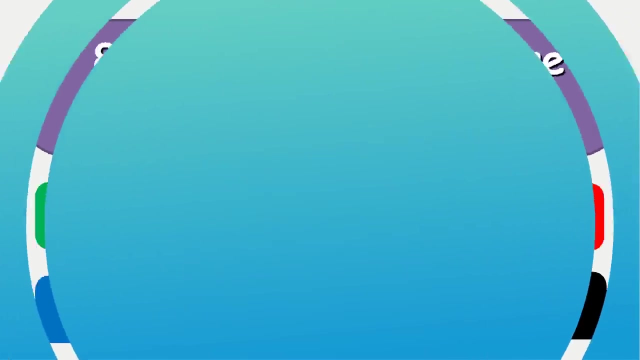 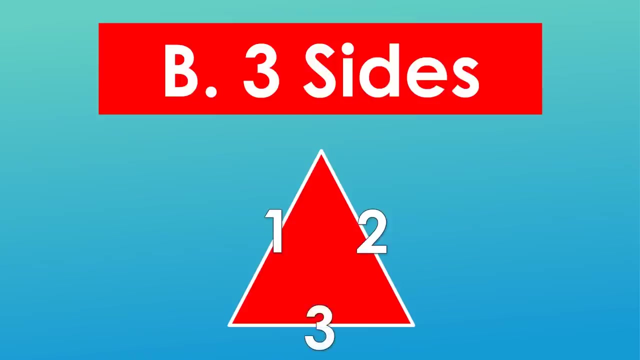 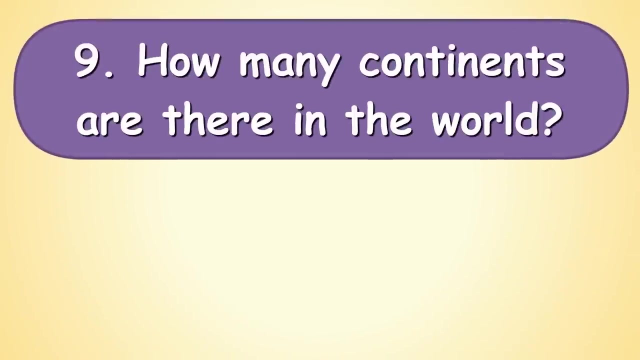 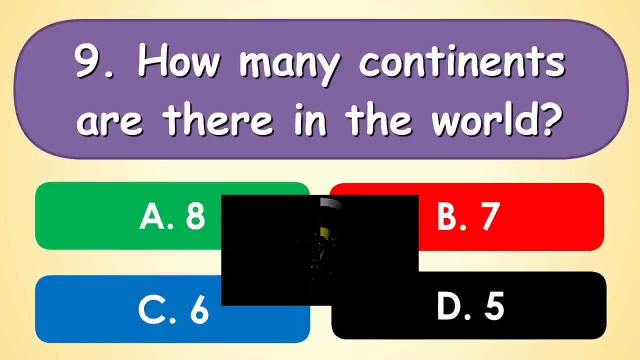 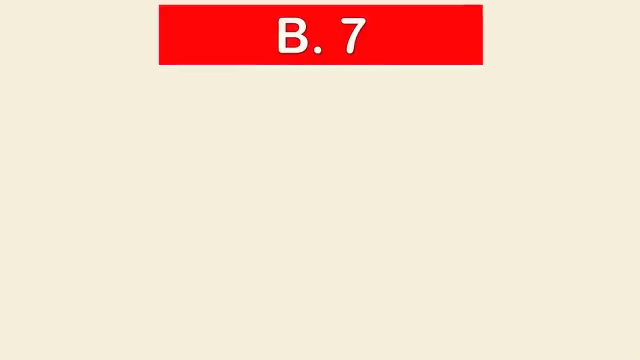 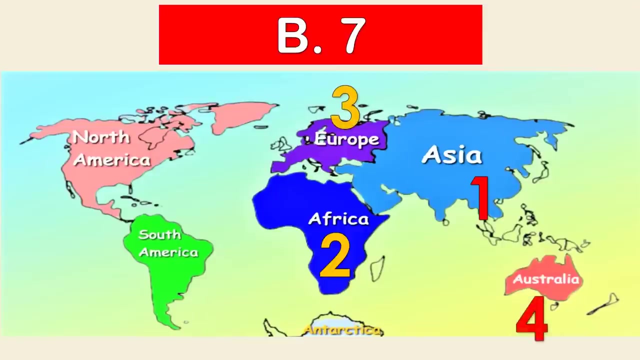 How many weeks are there in a year? 22 weeks. How many sides are there in a triangle? 3 sides: 1,2,3. A triangle has 3 sides. How many continents are there in the world? 7. Asia, Africa, Europe, Australia, South America, North America, Antarctica. 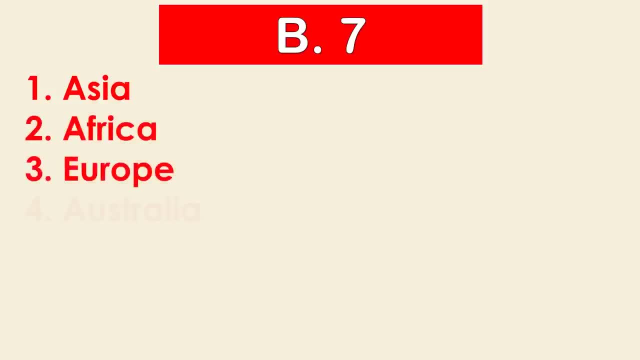 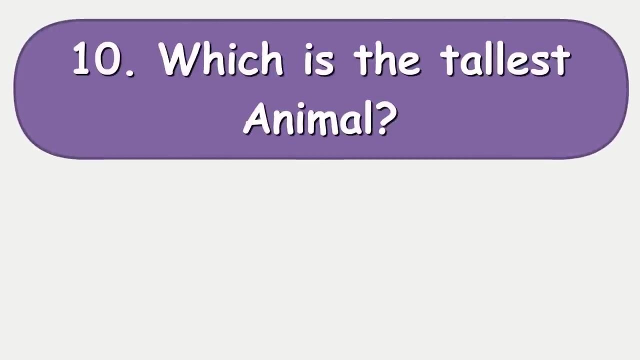 7 continents list are Asia, Africa, Europe, Australia, North America, South America and Antarctica, Which is the tallest animal, 6 continents ineren: East America, North America. North America waste media 입니다 10 continents in the universe. 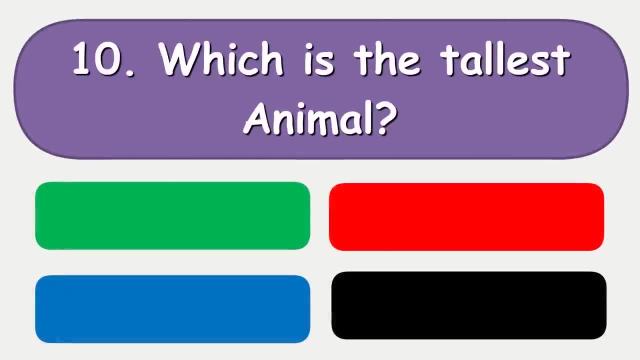 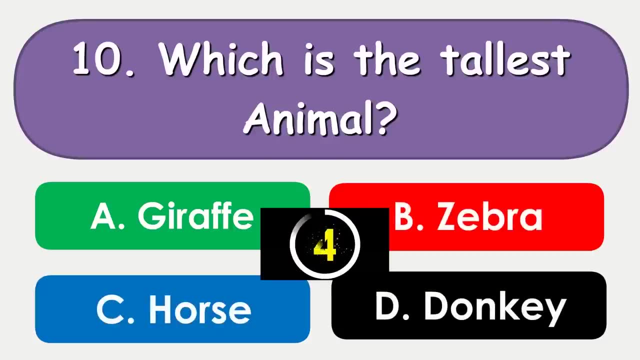 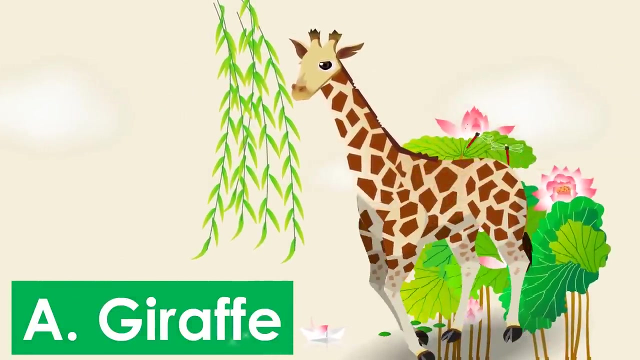 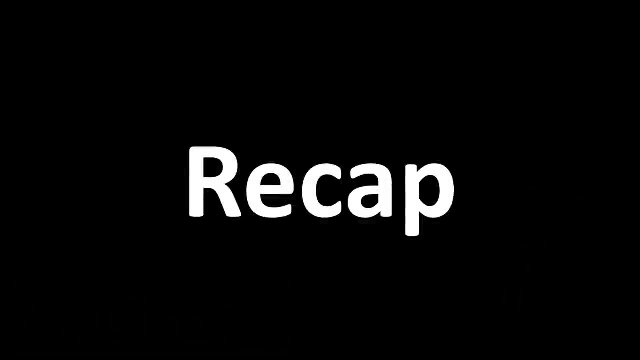 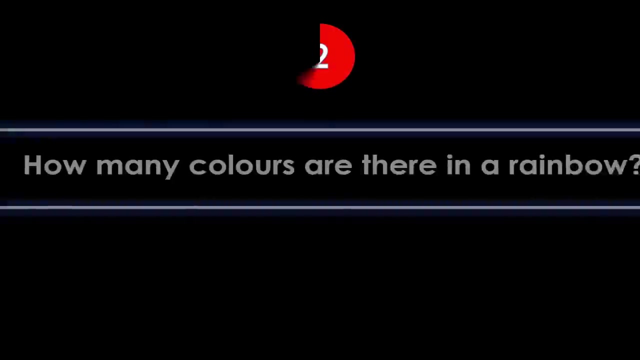 Which is the tallest animal? 3 continents, 4 continents on Earth, 3 continents in a year. Giraffe is the tallest animal. Recap the questions: How many days are there in a week? Seven days. How many colors are there in a rainbow? 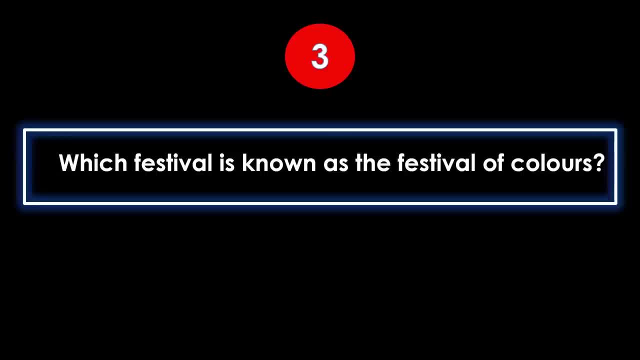 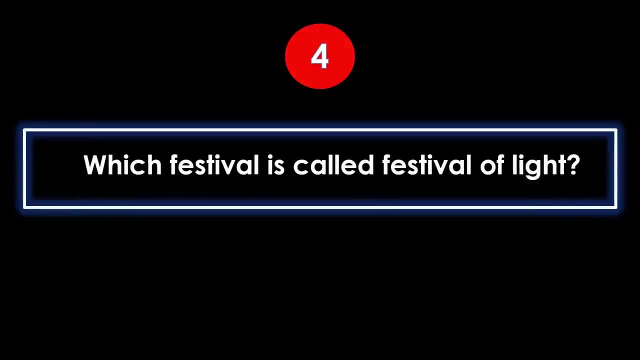 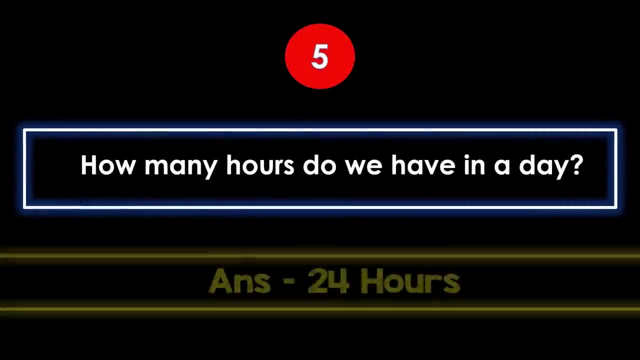 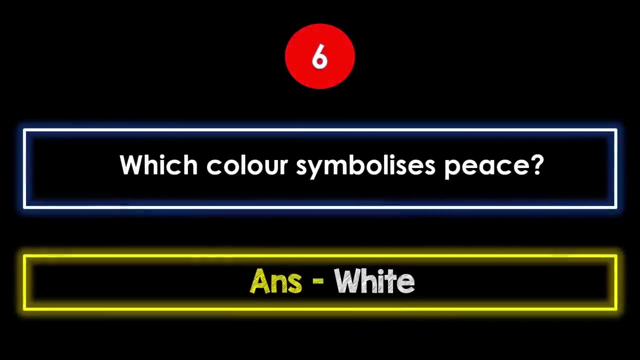 Seven colors. Which festival is known as festival of colors, Holi? Which festival is called festival of light, Diwali? How many hours do we have in a day? 24 hours. Which color symbolizes peace? White color. How many weeks are there in a year?